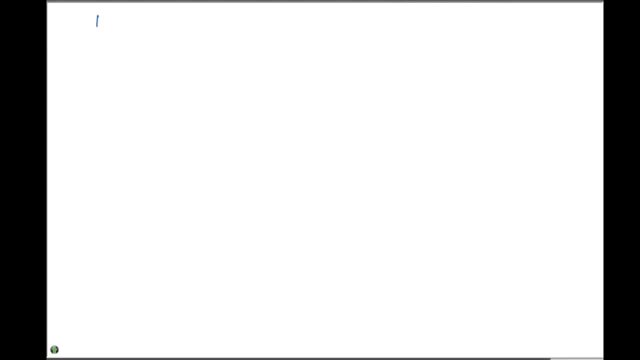 In order to do that, we need to look at bonding theories Of transition metal complexes, And the first theory that was introduced was something called valence bond theory, And this theory was more of an explanation than kind of a theory, And we basically stated that the metal acts as a Lewis acid, the ligand, 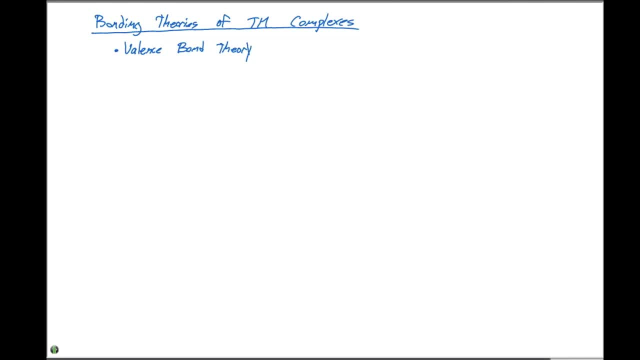 and so on and so forth. The ligand acts as a Lewis base, There's an attraction there and complexes form. It doesn't really go into the nitty gritty details of why particularly things happen, But we're having this sharing, or you know, of electrons forming these bonds. 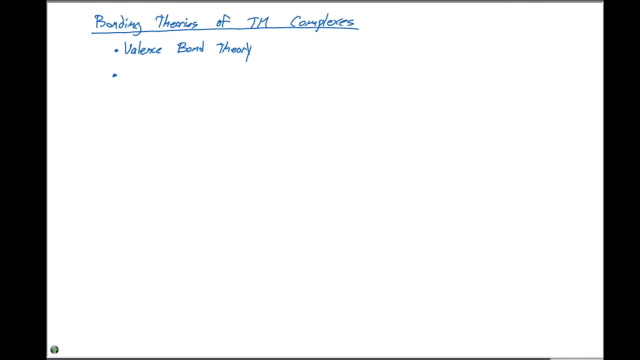 A more extensive theory is something called molecular orbital theory, And this basically extends on the theory that was shown in chapter nine of your textbook, Where you have these bonding molecular orbitals and anti-bonding molecular orbitals. The bonding molecular orbitals go down in energy. 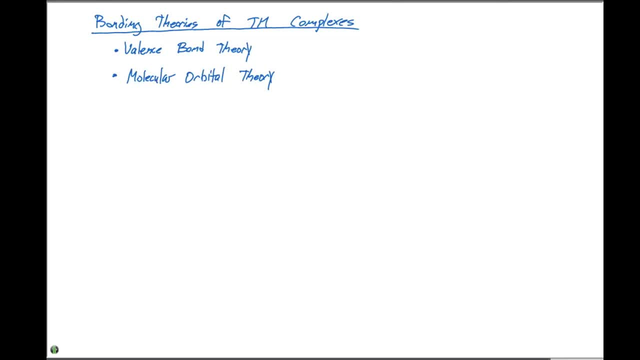 the anti-bonding molecular orbitals go up in energy. This theory uses advanced mathematical group theory. It's a lot of geometry type proofs And if you're really interested in this I would highly suggest you take chemistry 651, because we talk about group theory, probably in the first four weeks. 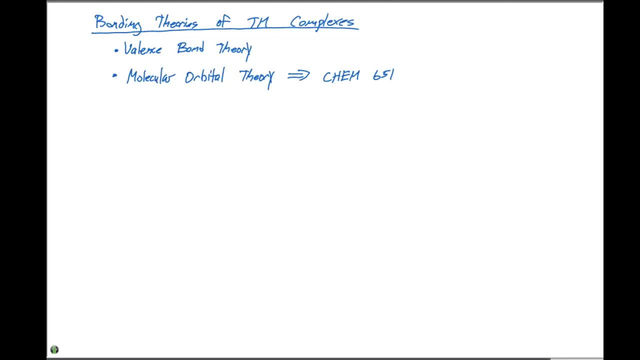 of that particular course. If you really wanna truly understand all the details of the color, you need to go into this theory. The problem is, if I tried to teach this class that, people's brains would probably explode. Right, It's crazy math. 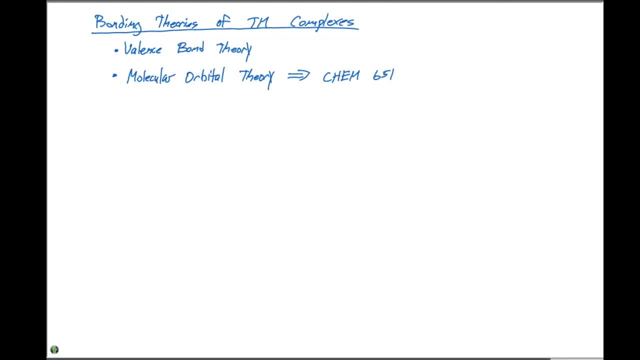 It's like good will hunting stuff where he's drawn out his little iterations right. So the question is, how can we take the relevant information from this molecular orbital theory and kind of make it relevant to a general chemistry class where we can teach all these concepts and kind of simplify the approach?